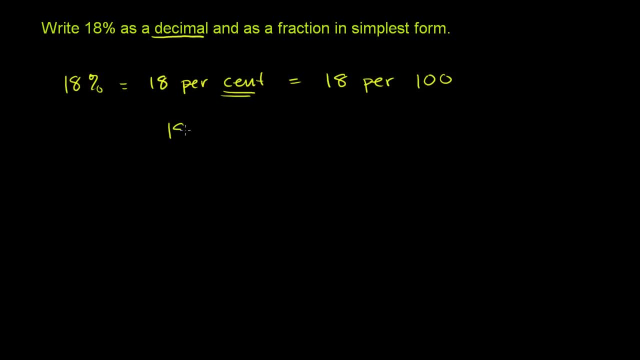 18 per 100 as a fraction literally means 18 per 100.. So we're doing the fraction first. This literally means 18 per 100, or 18 hundredths. Now, if we want to do it from here, we could go straight to a. 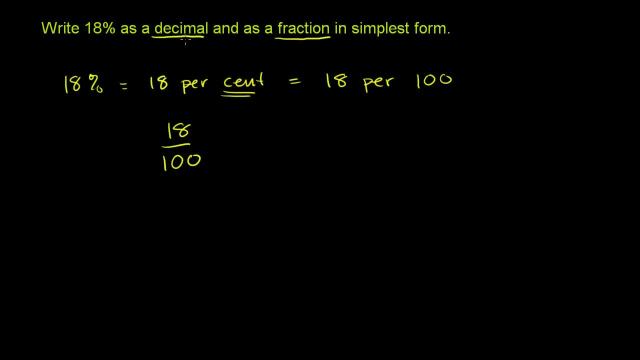 decimal. or we could do this fraction in simplest form: Let's do the decimal first, just because that's actually where I said I would do first. So let's do that first. So this is the same thing. This is the same thing as 18 hundredths. 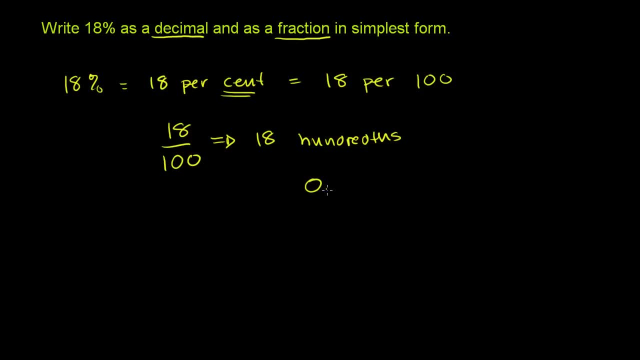 And we know how to write that. in decimal form It's 0.18.. You could view this as 1 tenth and 8 hundredths, which is the same thing, or 10 hundredths and 8 hundredths, which is 18 hundredths. 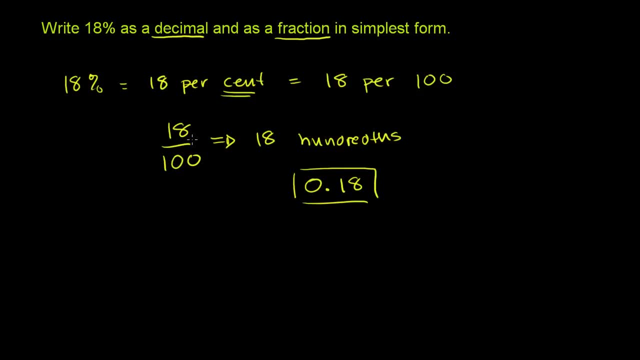 So this is written in decimal form And if we write it as a simplified fraction, we need to see if there is a common factor for 18 and 1 hundredth, And they're both even numbers, so we know they're both divisible by 2.. 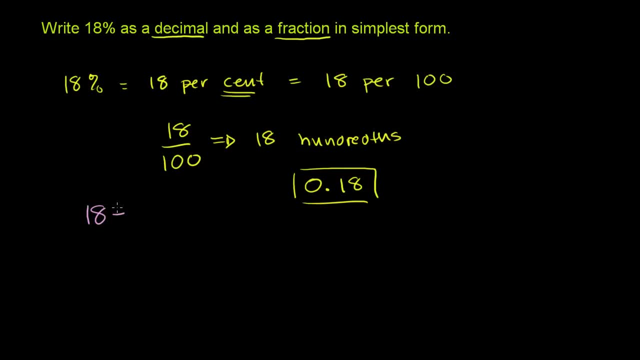 So let's divide both the numerator and the denominator by 2.. So we have 18 divided by 2 over 100 divided by 2.. And we're going to get: 18 divided by 2 is 9.. 100 divided by 2 is 50.. 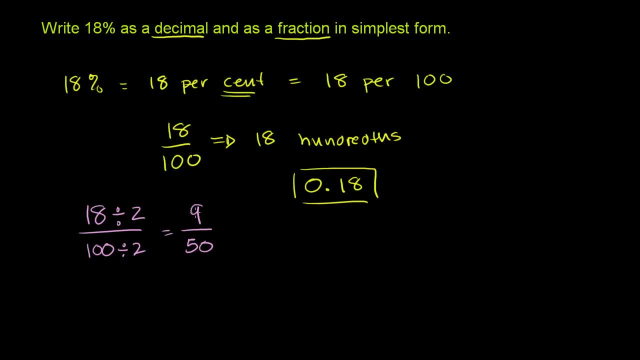 And I don't think these guys share any common factors. 50 is not divisible by 3.. 9 is only divisible by 3 and 1 and 9.. So this is the fraction in simplest form. So we have: 18% is the same thing as 0.18,, which is the 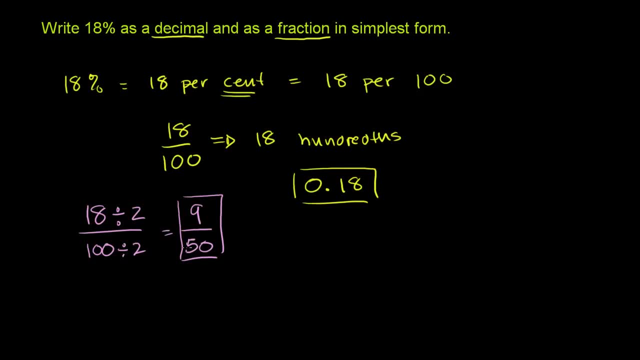 same thing in simplest form as 9 50ths. Now I went through a lot of, I guess, pain here to show you that, look, this really just comes from the word, from percent, from per hundred. But if you ever were to see this in a problem, the fast. 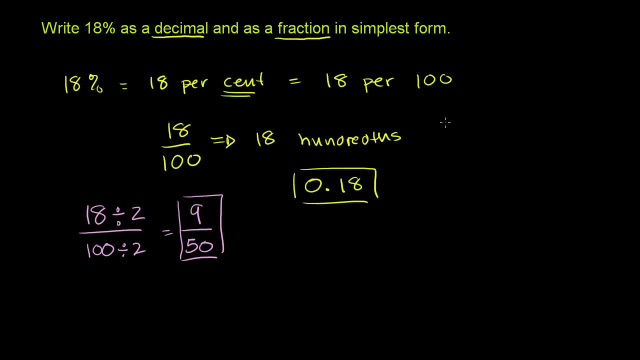 way to do this is to immediately say: OK, if I have 18%, you should immediately say anything in front of the percent. that's that anything, whatever this anything is, this should be equal to that anything. In this case, it's 18 over 100..